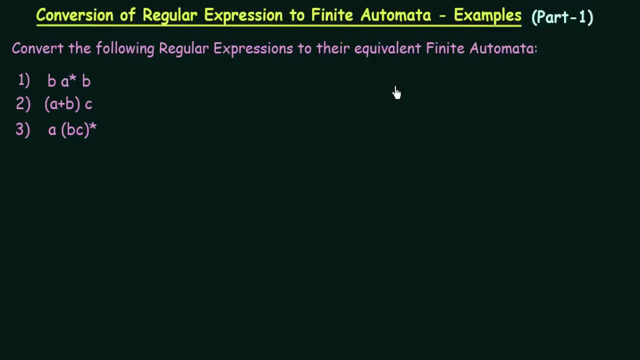 In the last lecture, I have taught you the rules that we need to remember for converting regular expressions to their equivalent finite automata. So in this lecture we will be using those rules and using those rules, we will be trying to convert these given regular expressions to their equivalent finite automata. 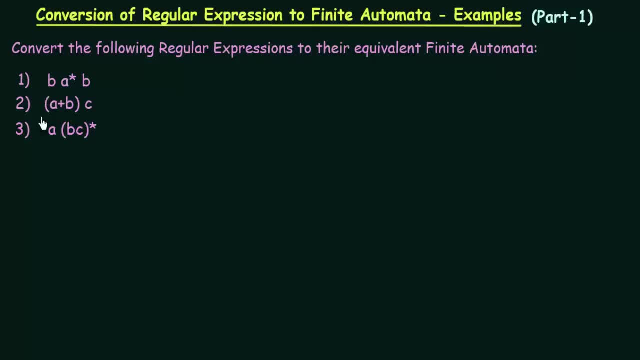 Okay, so let's get started. So here we have three expressions and we will start with the first one. The first one: it says b a, star b. So this means that the strings that will be accepted in these regular expressions are strings like b? b. 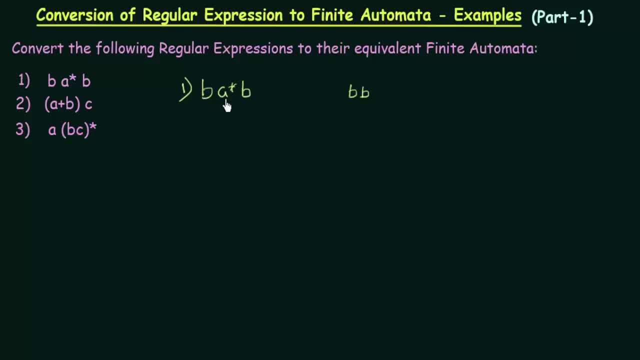 This means that it should have b followed by zero or more number of a's, which is a closure, and then followed by a b again. So here this b b means there is no a in between, Just b b, and it could also be b a b. 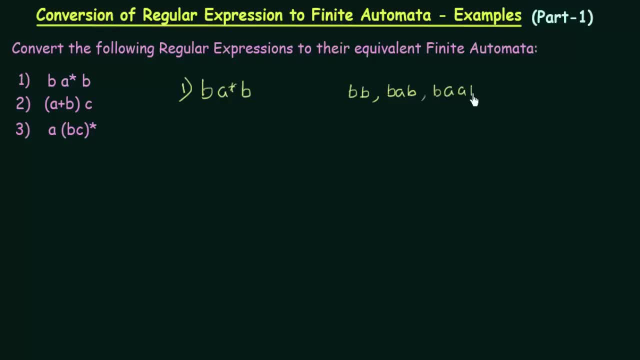 That means one number of a, then b, a, a, b and so on. So we need to design the finite automata for this. So I already taught you when the symbols are separated by, and. So what we need to do, Let me make the states. 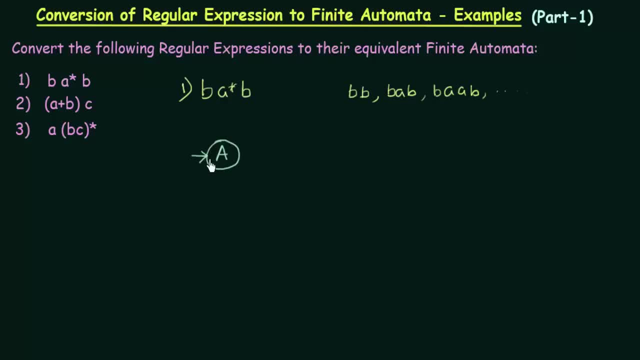 Let me say we have one state, which is state a, which will be my starting state, And I will have another state here, state b, And I will have another state here, state c And c will be my final state And I will say that this starting state a goes to b when it gets the input b. 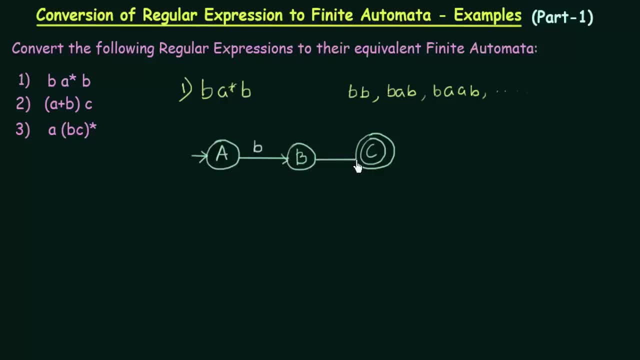 And then this b will go to the next state, that is state c, when it gets the next input b. So we have made for this b and this b. So what about this a? How shall we make for this a? I will make a self loop to this b itself when it gets the input a. 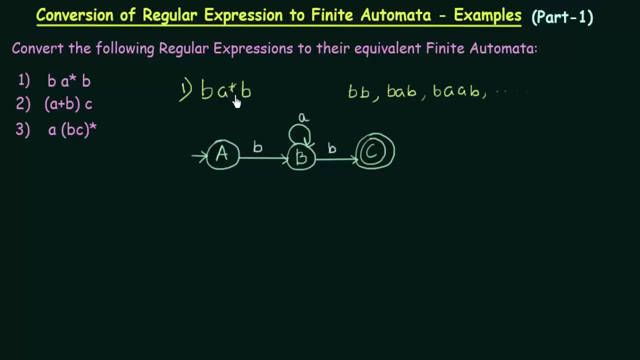 So I have already taught you in the previous lecture: whenever we have and operations, we have to make states for each of the input. So we have b and b here. They go to a, goes to b on getting input b, And b will go to the next state c when it gets the next input b. 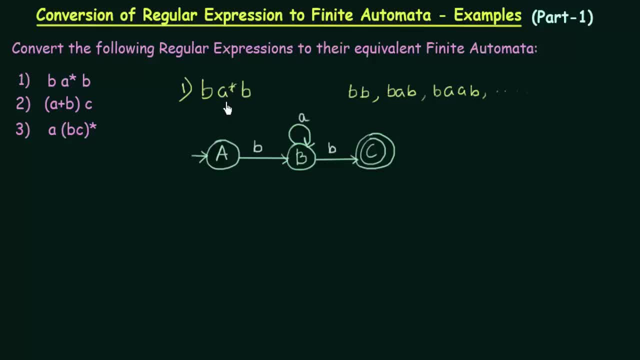 And whenever you have a closure of any symbol, you have to make a self loop. So here we have made the self loop in this state b. So let us check if these strings are accepted by this finite automata bb. So, starting from a and with b, it comes to this b. 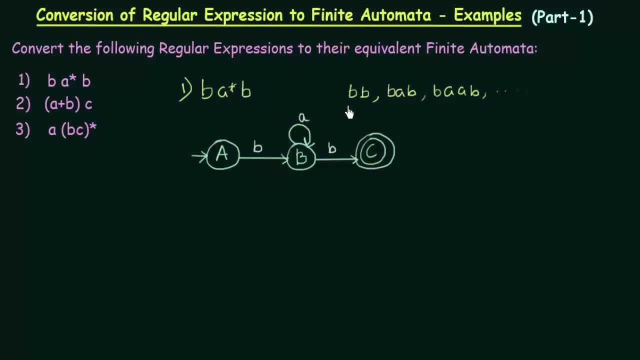 With the next b it comes to state c, which is the final state. So this is accepted. Now b, ab, b, ab, b again comes to the final state. This is also accepted. b, a, ab, b, a, another a and then b comes to the final state again. 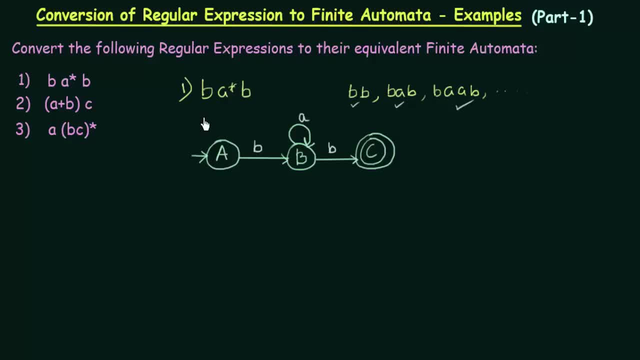 This is also accepted. So now we have successfully designed the finite automata for this regular expression: b a, star b. Okay, now let us go to the second one. So the second one says a plus b And then followed by a, c, like this: 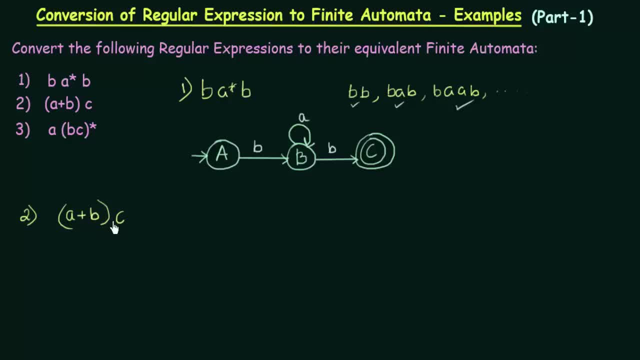 So here we have a union or a plus operation, and here we have a and operation. So in this case, what shall we do? I already taught you in the previous lecture that whenever you have a plus symbol, you can treat it as a or. 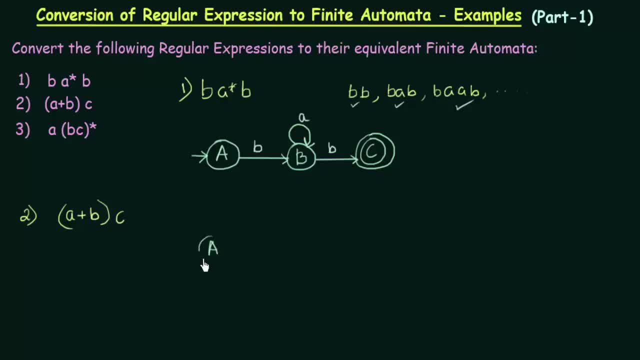 So let us say I have a state a, which is my starting state, And I will have the next state, which is state b, And then a can go to the state b. So a can go to the state b on getting input a and also a can go to the next state b even on getting the input b. 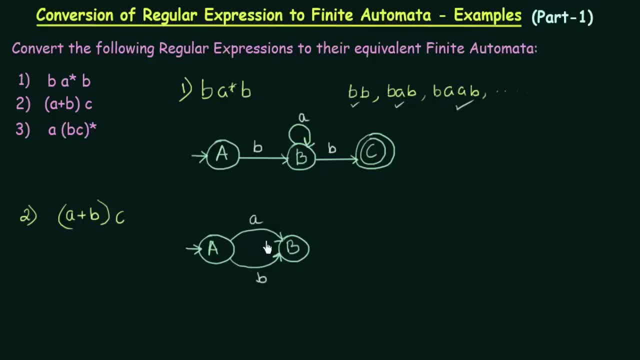 So whenever you have a plus symbol in between them, this is the way you make it, So a can go to the next state, b on both inputs a and b, And now we have the next input, c, And this should proceed to the next state. 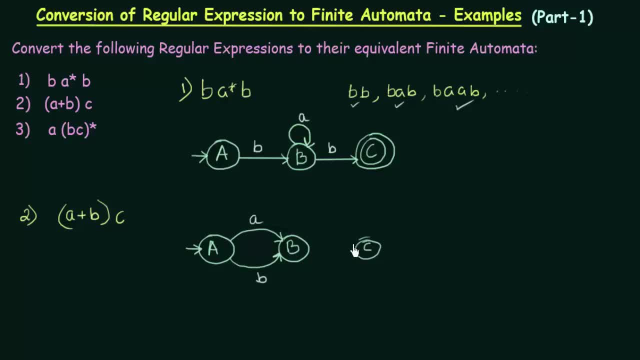 So this is the next state, which will be my final state. c, And when does it proceed On getting the input small c? So this is the finite automata for this regular expression. So let us see what are the strings that are accepted by this regular expression over here. 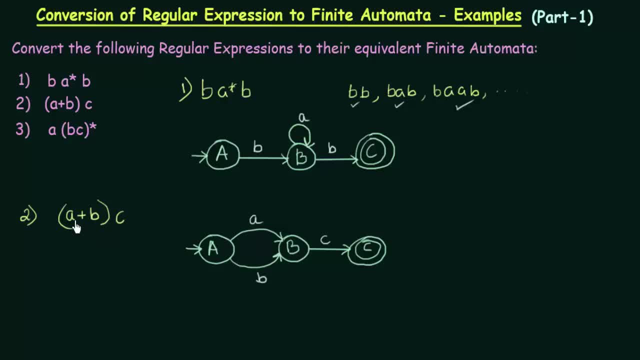 So a plus b and c. So that means a or b followed by a c. It could be a followed by a c, Or it could be b followed by a c. So these are the kind of strings that will be accepted by this regular expression. 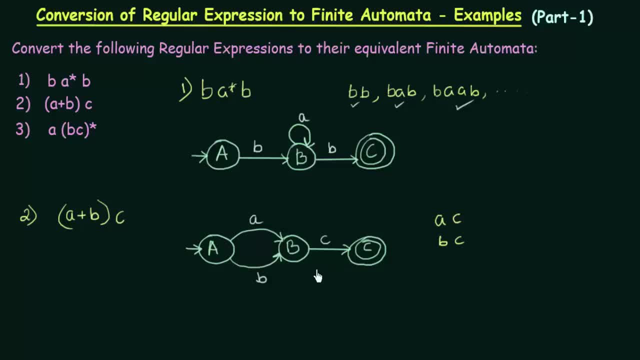 So let us see if this is accepted by this automata that we have created. a- c comes to the final state. This is accepted. b- c comes to the final state. This is also accepted. So we have successfully designed the final automata for the regular expression a plus b and c. 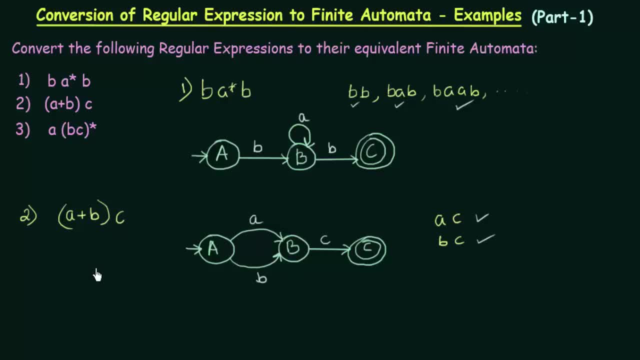 All right, So we are done with that. Now let us come to the next one over here, Number 3, which is a, and in bracket I have b c star. Okay, So before we design the final automata for this, 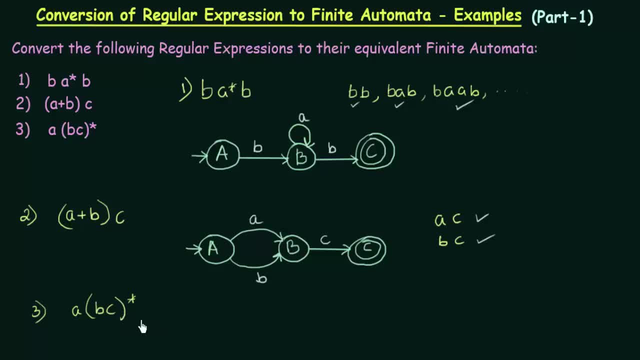 let us see what are the kind of strings that are accepted by this regular expression. So this means that a and b c closure. That means a followed by any number of b c. This group b c- can be 0 or more, So it may be like a just by itself, because I said b c could be 0 or more. 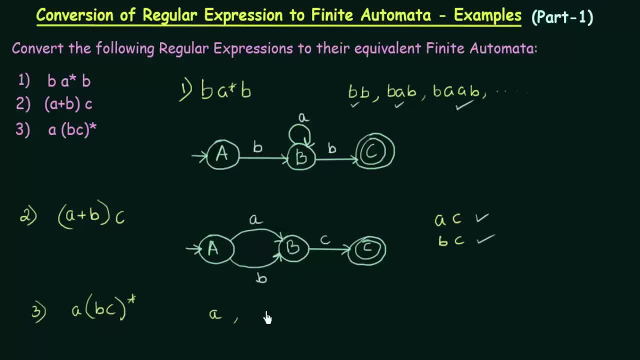 So if b c is 0, then it could be just a or it could be like a b c. That means 1 b c. or let us say a b c, b c, Right, 2 b c's, or a b c, b c, b c. 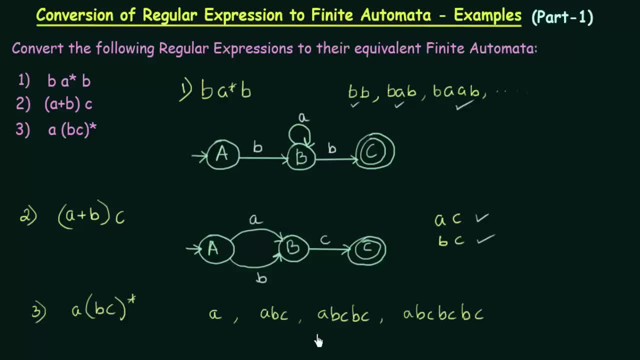 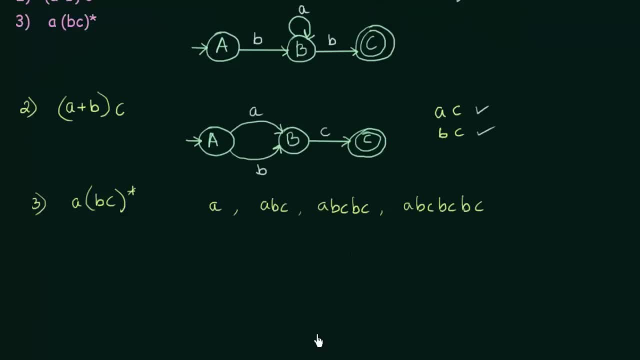 3, number of b, c's. So these are the kind of strings that will be accepted by this regular expression. So let us see how we can design the final automata for this. So I will start with a state, which I will call state a, which will be my starting state or initial state. 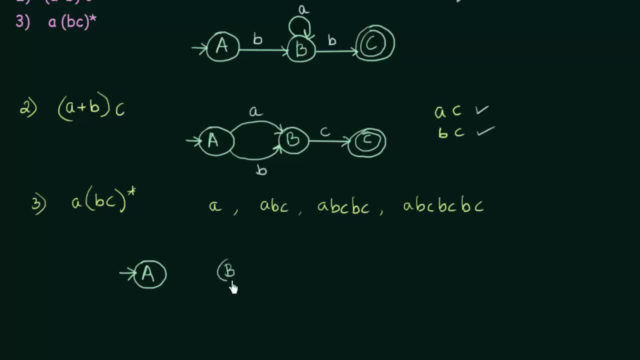 And I will make another state here, b And I will say that a will go to the next state b on getting input small a. Okay, So we are done with this part. Now I need the closure of b c. So in order to make the closure of b c, I will make another state here, which I will call state c. 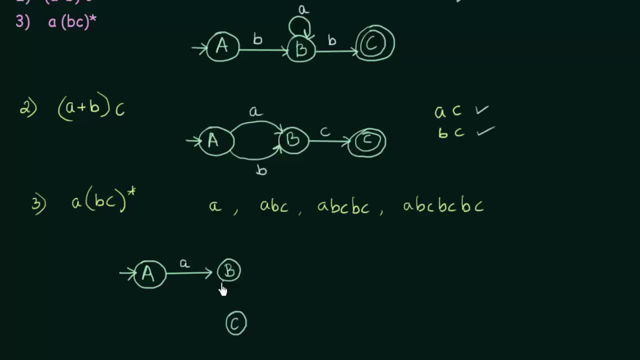 And I will say that from state b it will go to c on getting input small b, And from c it will go back to state b on getting input small c. And here what will be my starting state And here what will be my final state. 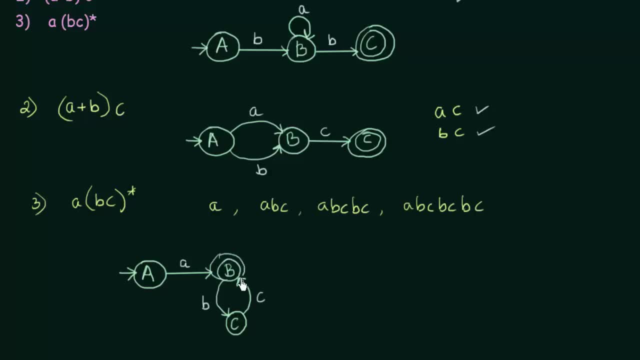 I will make b as my final state. Now, why did I do this? This is because we see that whenever we reach b, c, whenever c is the last symbol, that is when the string is ending, or that is the string set- will be accepted. 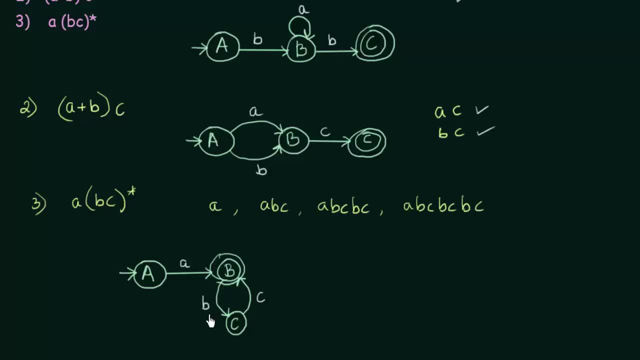 So here we see that when it gets input small b it comes to c, But c is not a final state. But when it gets the input small c- See like here- It goes to b, which is a final state. And also the string a by itself also should be accepted. 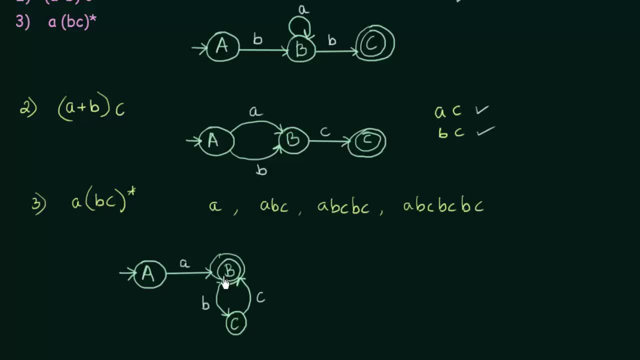 That is why it comes to this final state b when it gets input small a. So let us just check if these strings are accepted or not. a by itself. a by itself: It comes to the final state b: It is accepted. 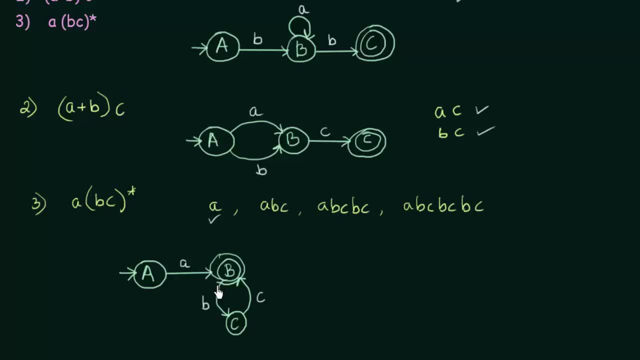 a, b c. So a, b and c again comes to the final state: accepted: a, b, c, b c, a, b c, again b c. accepted a b c, b c, b c. 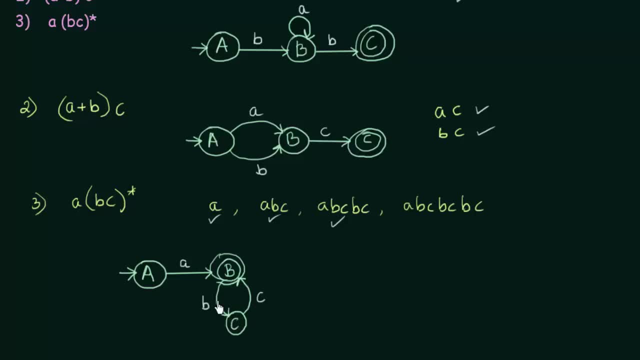 a, b c, b c, b c. So any number of b c's that you have, it will be accepted. So now we have also designed the finite automata for this regular expression. So this is how you convert the regular expressions to their equivalent finite automata. 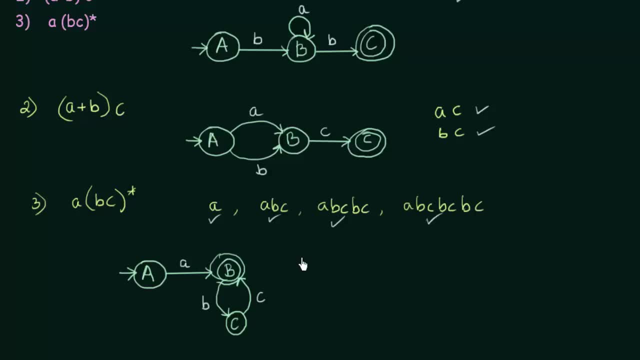 And we will be seeing more and bigger examples in the coming lectures. So thank you for watching and see you in the next one. 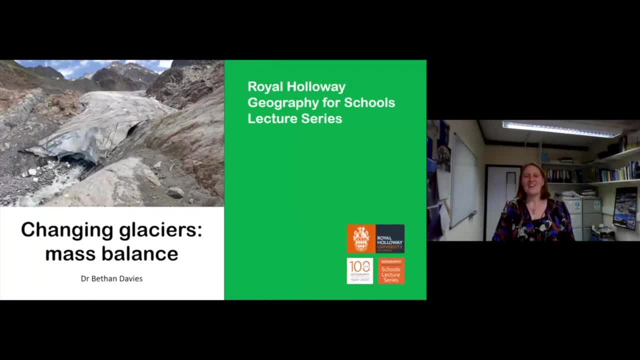 Hey, hello, Welcome to this Jog FIFA Schools lecture on changing glaciers and glacier mass balance. In this lecture, I will be talking about what is glacier mass balance and how it is changing across the world today, and what that means in terms of water resources for the people that depend on these glaciated mountains.